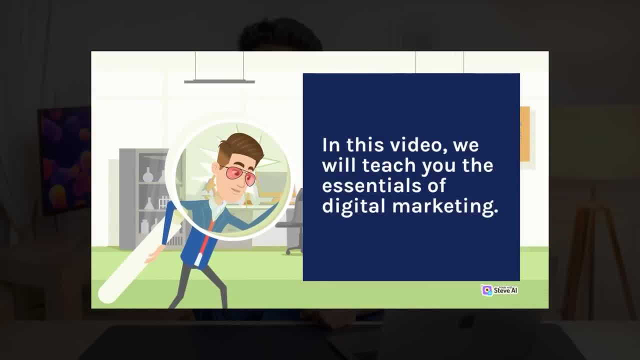 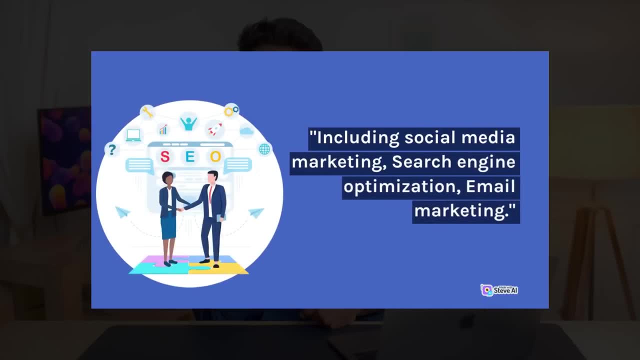 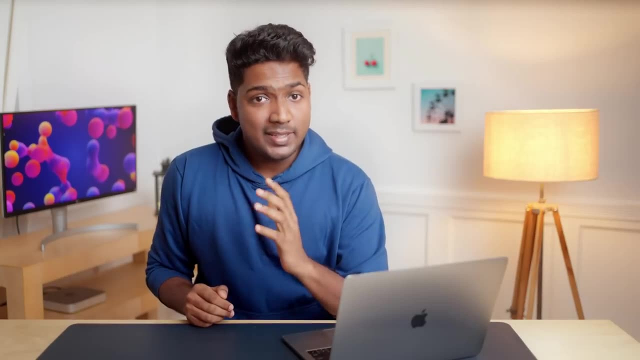 marketing in five minutes. In this video, we will teach you the essentials of digital marketing, including social media marketing, search engine optimization, email marketing, So make sure you watch this video till the end. I'm Brian from Website Learners, and let's get started. So, to make the animation video, we are going to do two steps. 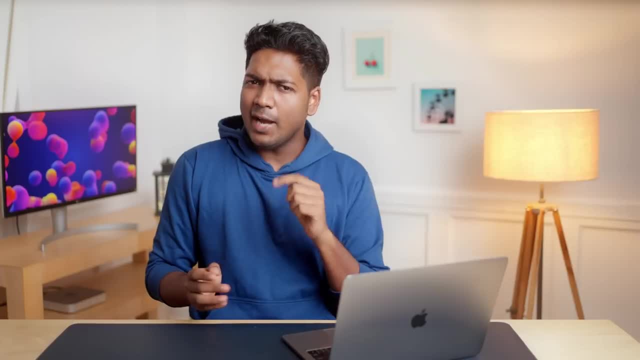 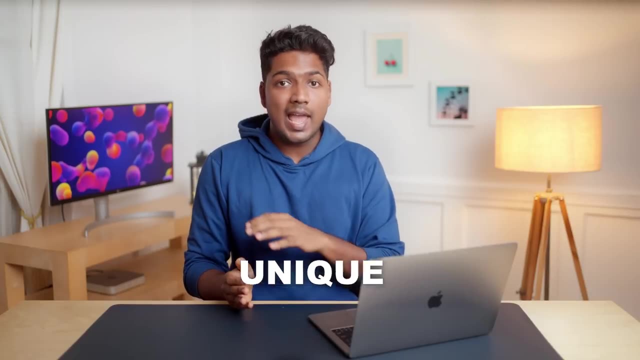 The first step is to generate the script. I know a fantastic tool called Gravity Write which will help us do just that. Gravity Write lets you generate high quality, unique and creative content for various purposes, like websites, blogs, video scripts and more. 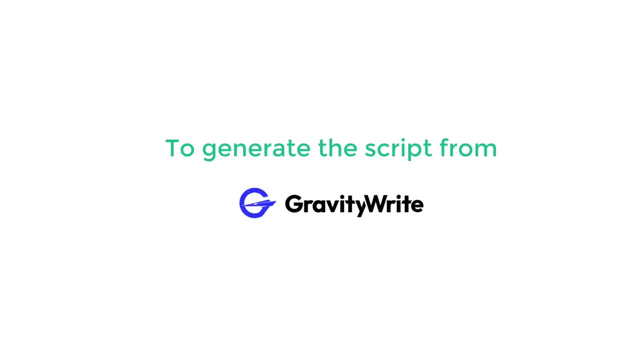 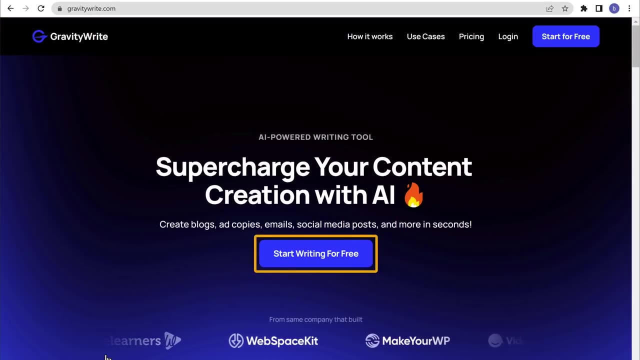 Okay. so to generate a script from Gravity Write, we need to create an account on it. So to create an account, just click the link below this video and it'll take you to the site. Now click on Start Writing for Free Here. enter your details. And, after entering your details, 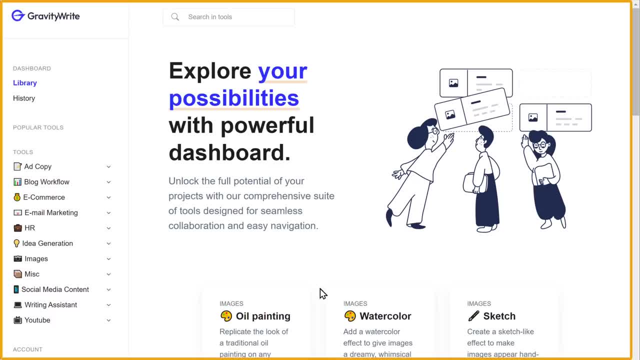 and then click Create Account and it'll take you to the Gravity Write dashboard, which means we have created an account on Gravity Write. Once you have created your account, you will see that you have created an account on Gravity Write. Once you have created your account, you will see that you have created an account on Gravity Write. 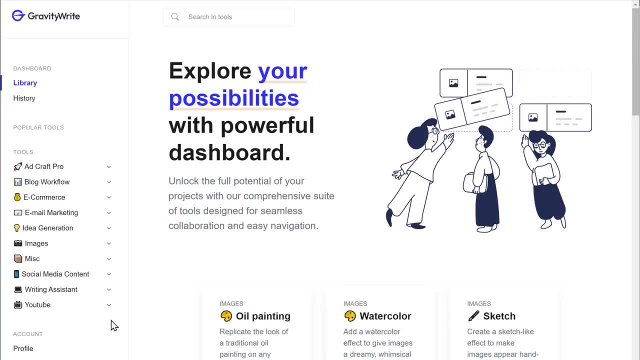 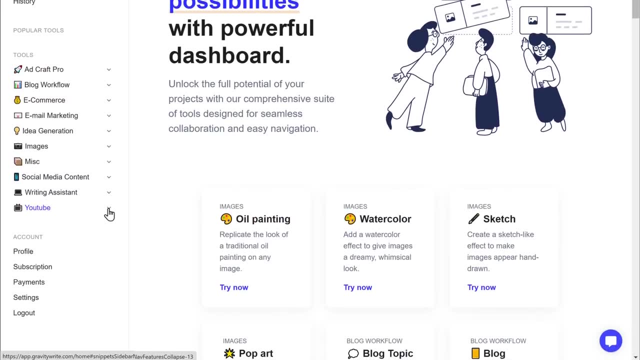 your account. next we need to generate the script. for example, let's say you want to create an animation video to promote your products or services, so all you have to do is just go to the youtube option, then click on explainer video script here, enter these details and generate the. 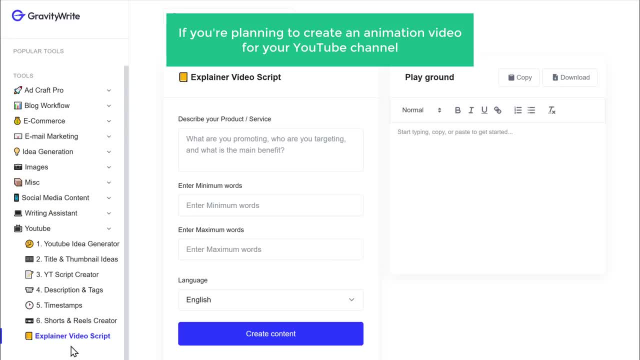 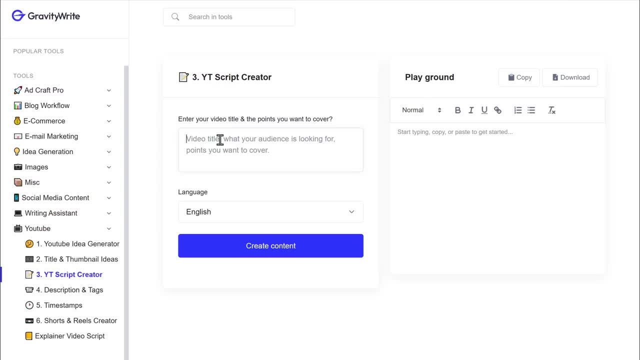 script. or if you're planning to create an animation video for your youtube channel, just click yt script creator and here you can generate your script. for that you need to enter your video title here. so i'm going to enter: learn digital marketing in five minutes, then type a few. 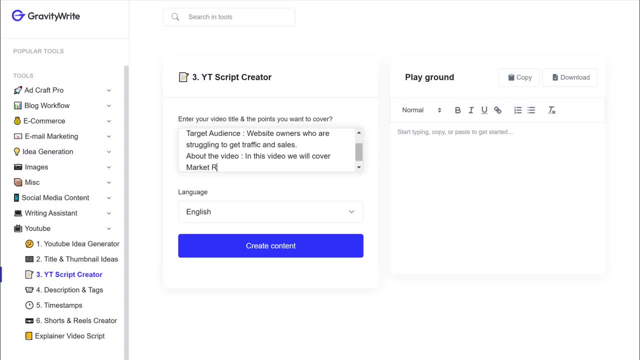 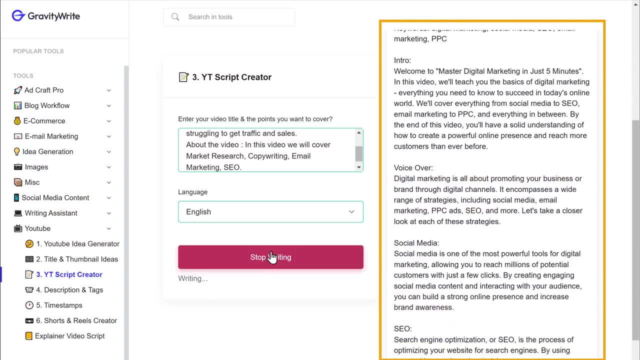 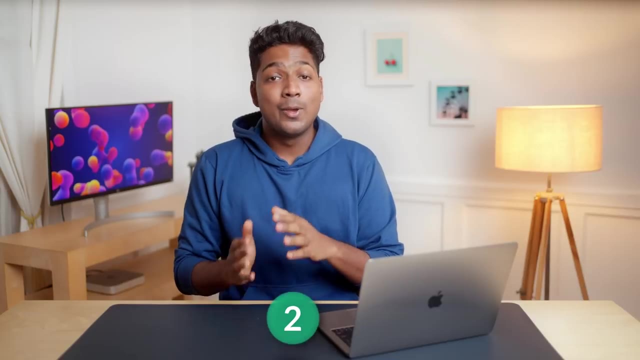 lines about what your audience is looking for, and then enter the points that you want to cover in the video. once you are done, click create content and you can see that the script has been successfully generated. we can now go to the second step, which is to convert this complete script into an 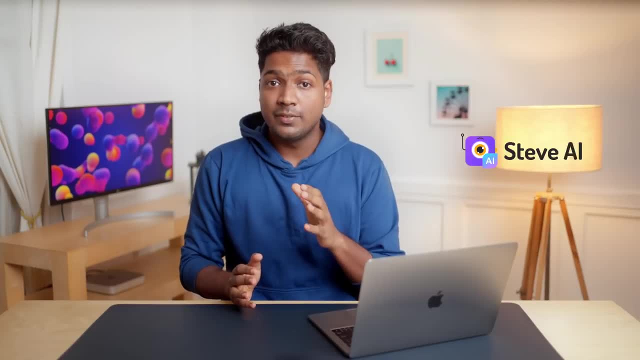 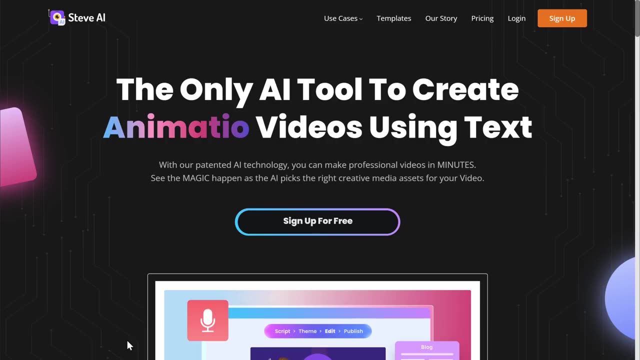 animation video. to do that, we are going to use a tool called steveai. first we need to create an account on steveai. so to create the account, just click the link below this video and click sign up for free. now simply sign up with google. 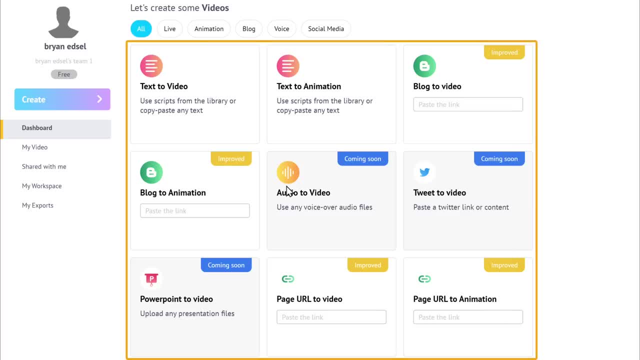 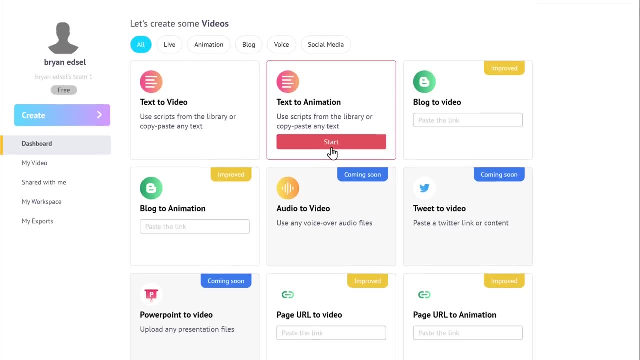 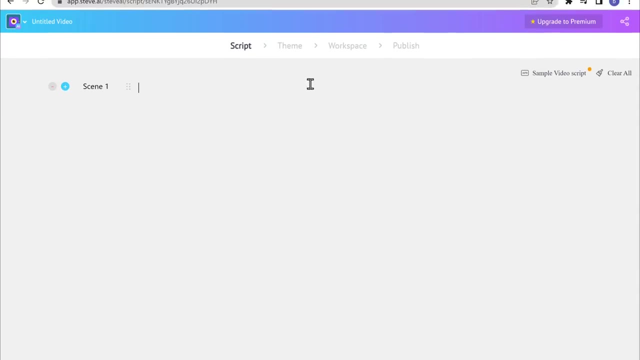 and it will take you to this dashboard. here you can see we have different options. as we want to convert our script into an animation video, let's choose this option and it will take you to this page. now, here we need to paste our script, which we generated from gravity right, so let's go to. 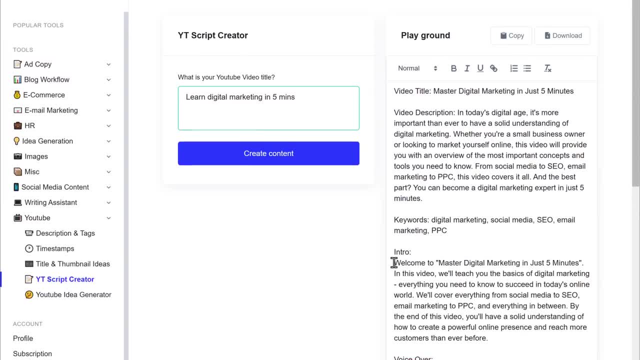 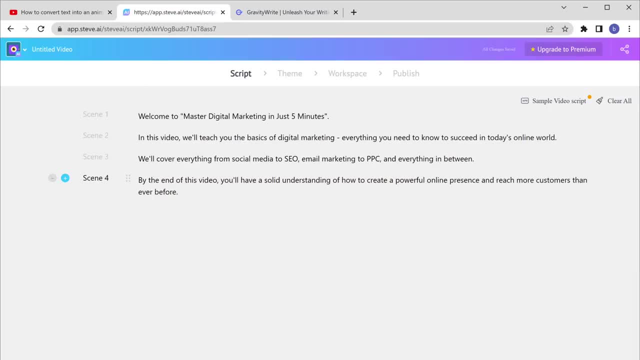 the page, and here you can see the script that we generated earlier. first we will copy this intro part, then go back here and paste it. now, as you can see, the script has been converted into different scenes. in the same way, we will copy the remaining parts and 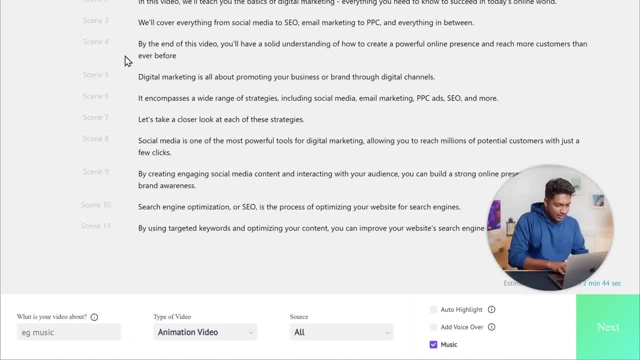 let's paste it here. so once we have pasted the script here, you need to enter what type of video it is. so let's click here and enter the type of video. once you have entered that, click next. now you need to select the design for your video. so if you place the mouse pointer on any design, 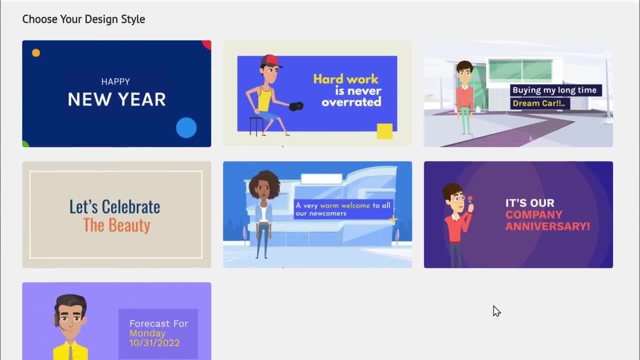 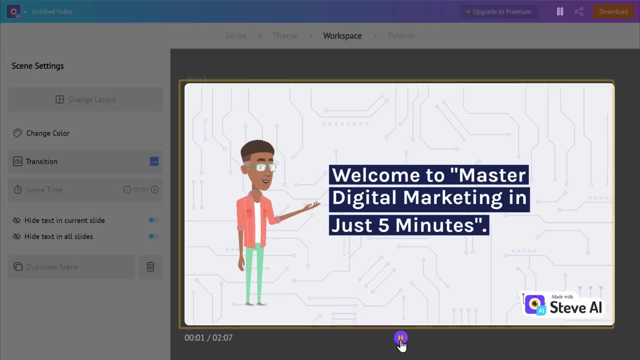 it will show you the preview and you can choose any design you like, so i'm going to choose this one now. if you click play, you can see that it has converted an entire script into an animation video. if you want, you can make changes to this animation too. 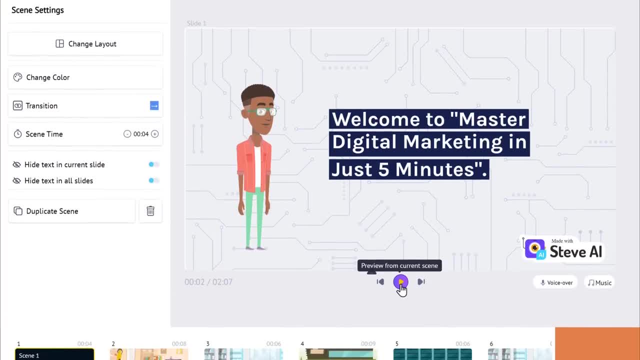 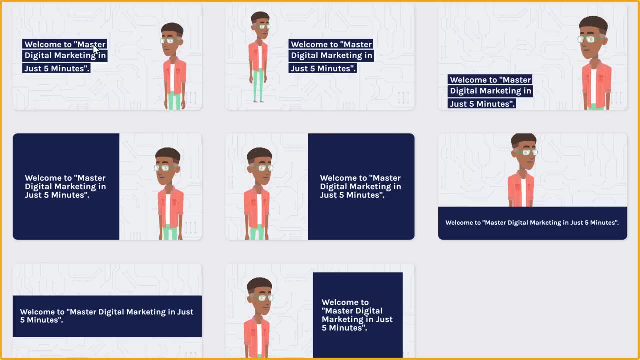 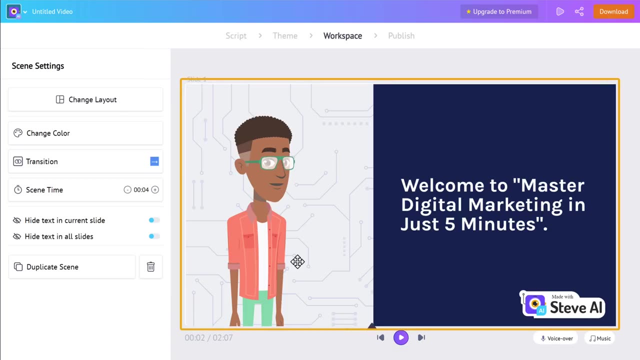 we'll also be able to edit each scene individually. so first let's see how you can change the layout of the scene. so just click here and you can see that we have got different layouts to change to. you can choose any layout you want. i'm going to choose this one and you can see that the new 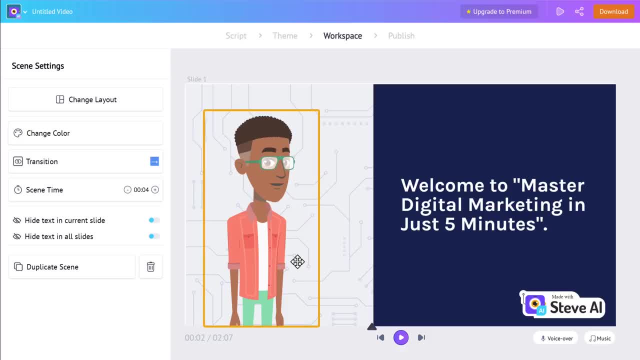 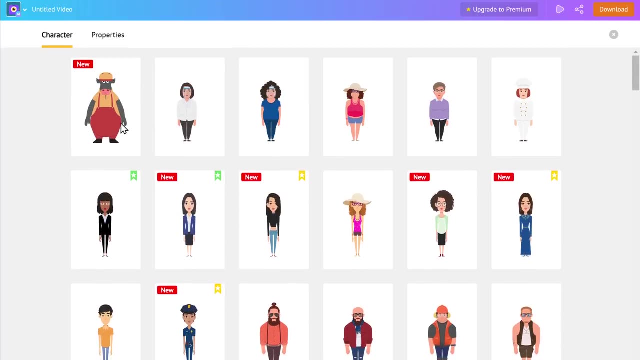 layout has been applied to our video. okay, let's say you want to change this character into another character, so all you have to do is click on it and you will get different options. now click on change character and you can see that we have got different characters to choose from. i'm going to choose this one. 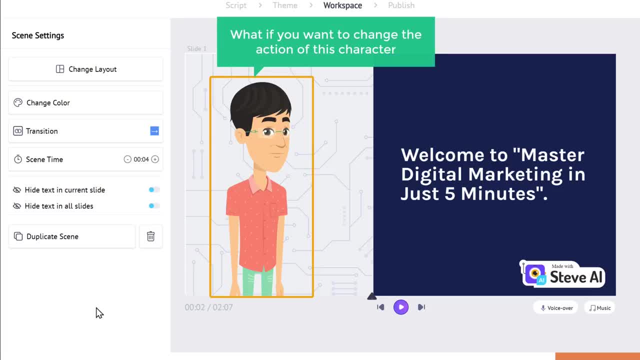 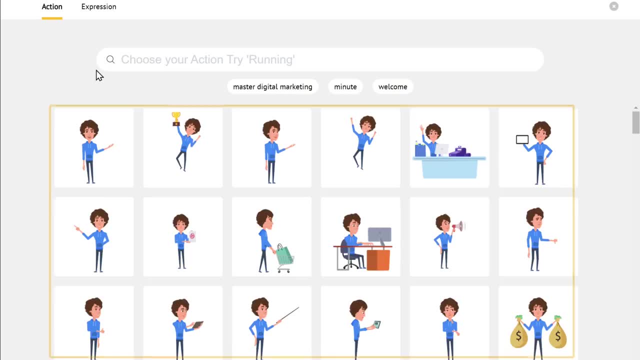 as you can see, the cat has been changed in the scene. now what if you want to change the action of this character? you can do that by selecting the character, then click on change action and you will get different actions to choose from, so you can choose the one you want. 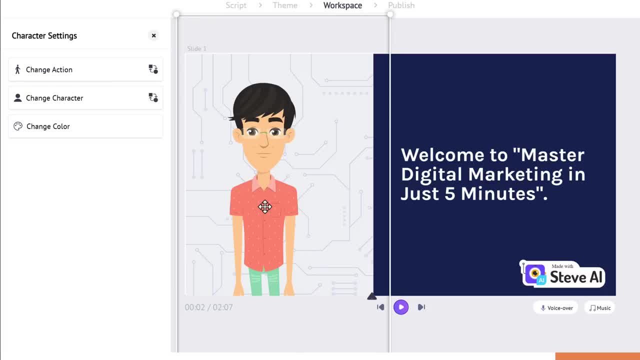 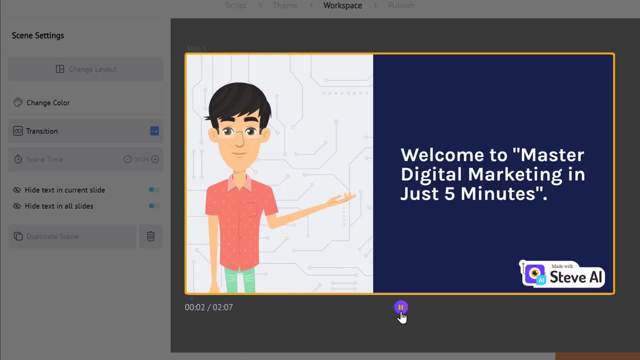 and it will be applied to the scene. also, you can move the position of the character like this and keep it wherever you want. if you play the video, you can see that the changes have been applied, and now we have learned how to change the layout and the character. next let's see how you can. 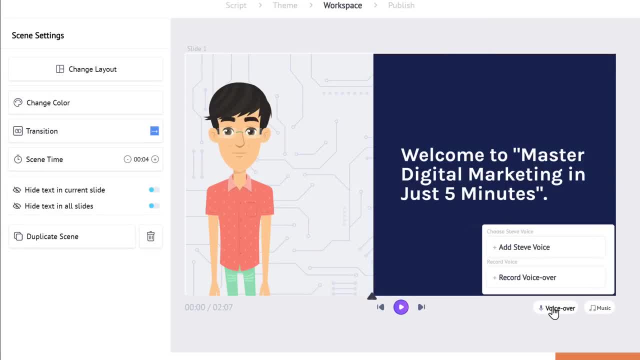 change the layout of your voice over to your animation. to do that, just click here and you will get two different options. you can either add an ai voice or record your own voice. i am going to add an ai voice, so let's click here and you can see that we have got these options to choose from. so for the ai, 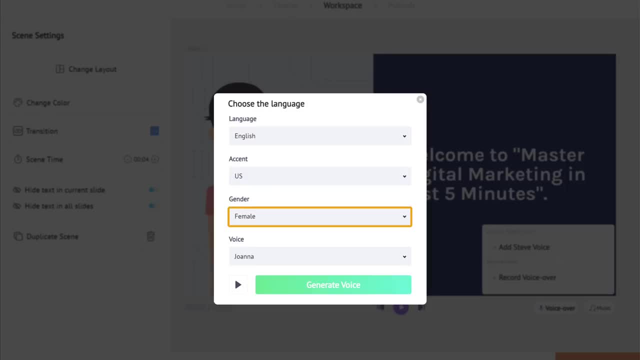 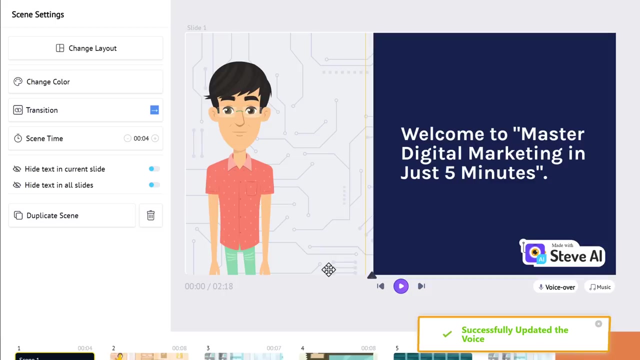 voice. you can choose the language, the gender and also select the voice you want. now, if you click here, you can hear a preview of the voice. hello, i am matthew from steve, and once you're happy with this, click generate voice and the ai voice will be generated and applied to your video. 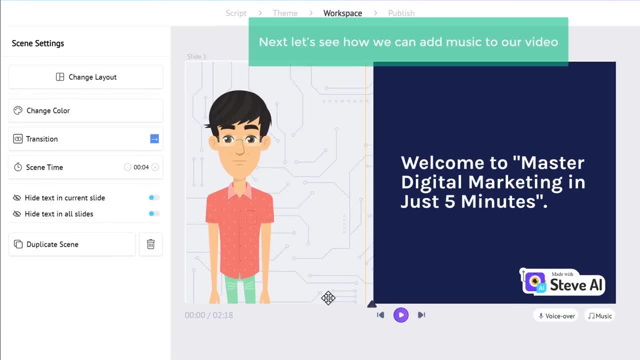 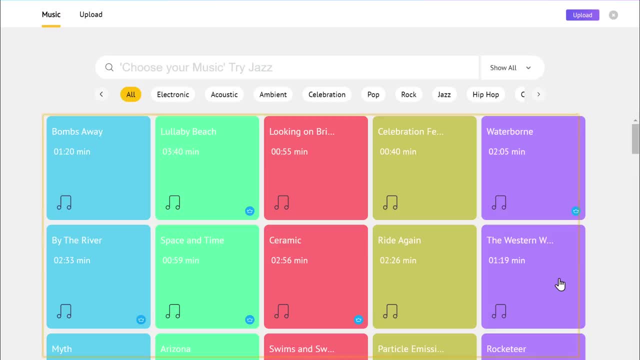 so this is how you can add an ai voice to your animation video. next, let's see how we can add music to our video. so to do that, let's click on music. then click here and you will get a lot of different music to add to your video. if you place the mouse on any music here, you can. 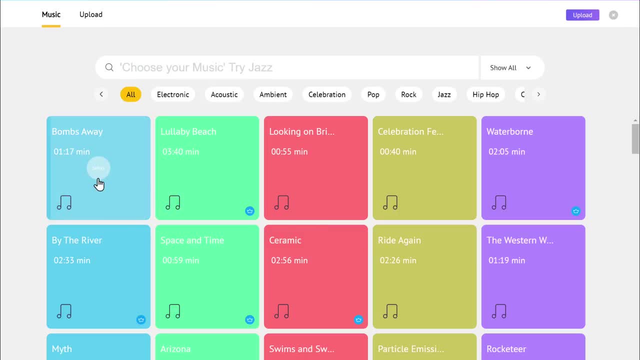 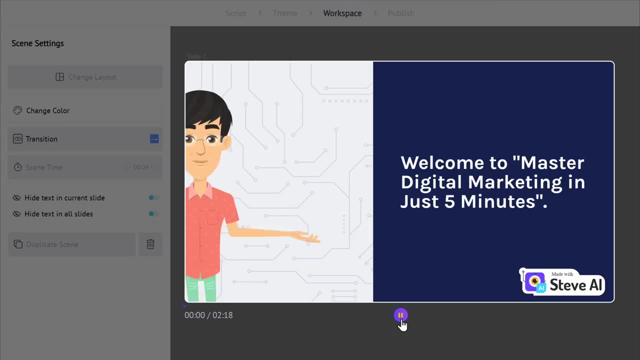 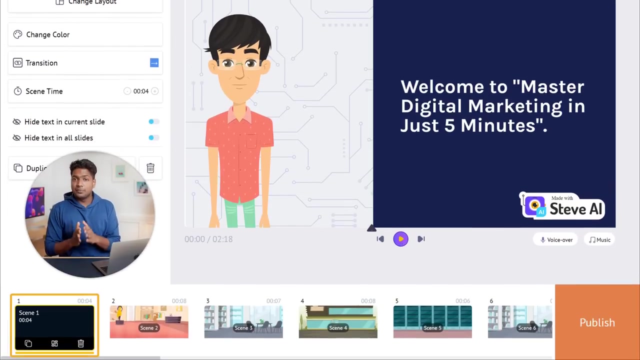 hear the preview and if you like the music, you can add it to the video by clicking on it now. if you play the video, welcome to master digital marketing. in just five minutes you can see that the music has been added. okay, so now we've edited the first scene. 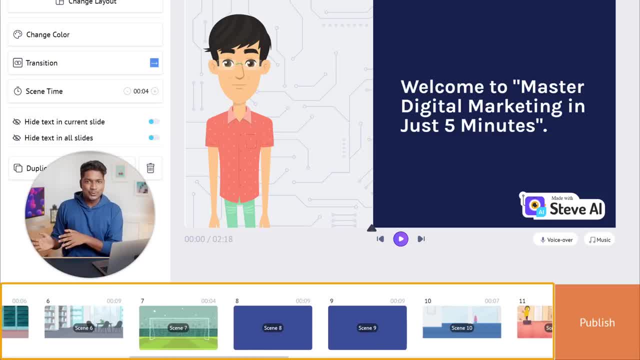 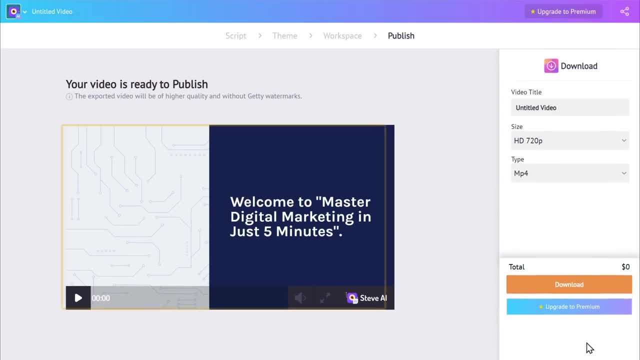 of our animation video. in the same way, we can edit all the other scenes too. so once you're happy with your video, let's download it. so to do that, just click publish. as you can see, our video is now ready to download. now, if we click download. 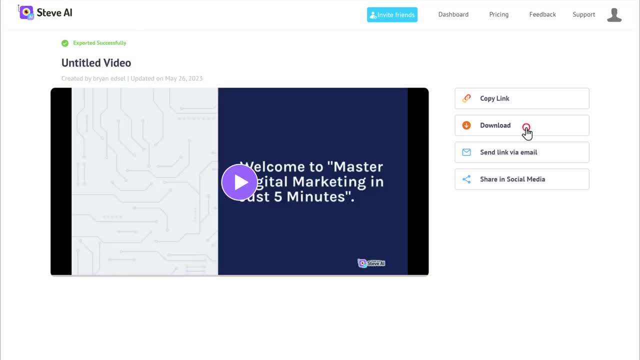 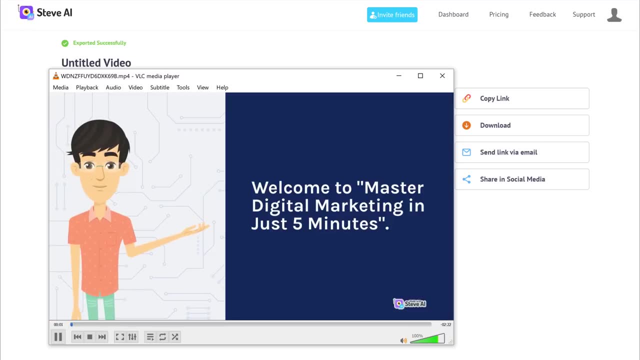 your video will be exported here and again. click download here and you can see that Our animation video has been downloaded to our computer Now if we open it, Welcome to master digital marketing in just 5 minutes. In this video, we'll teach you the basics of digital marketing. 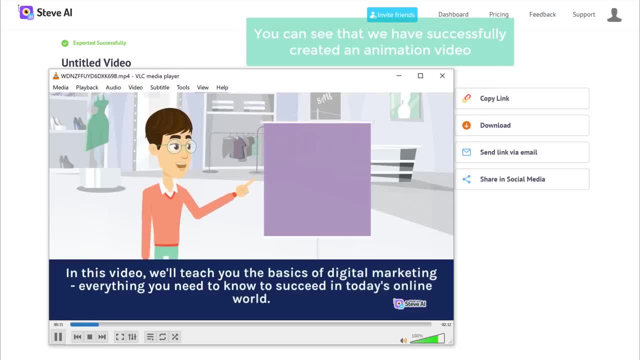 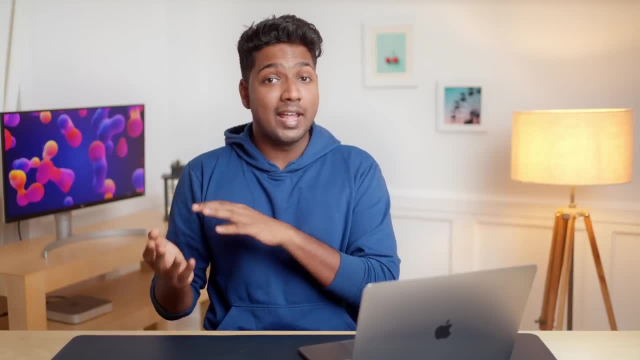 Everything you need to know to succeed in today's online world. You can see that we have successfully created an animation video. In the same way, you can generate scripts for your videos from Gravityrite And then convert the same script into an animation video. 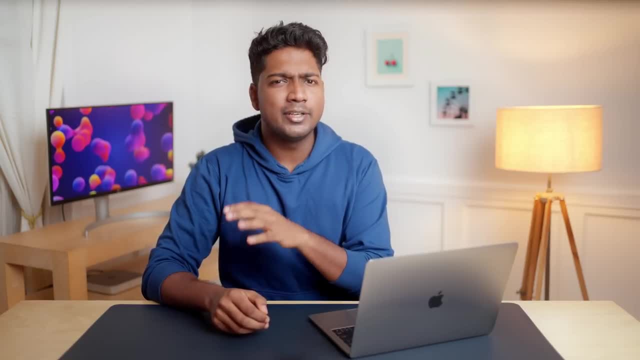 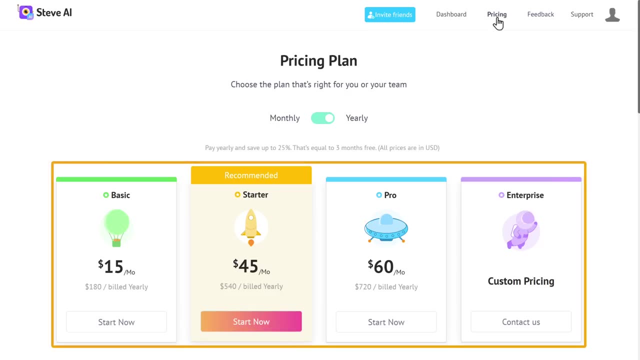 Okay. using the free version of Steveai, you can create and download only up to 3 videos per month. So if you want to download more than 3 videos, you can click here and upgrade it. Okay, so now you know how you can convert your script into an animation video. 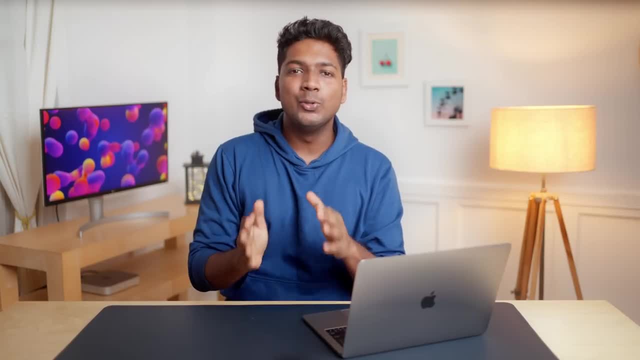 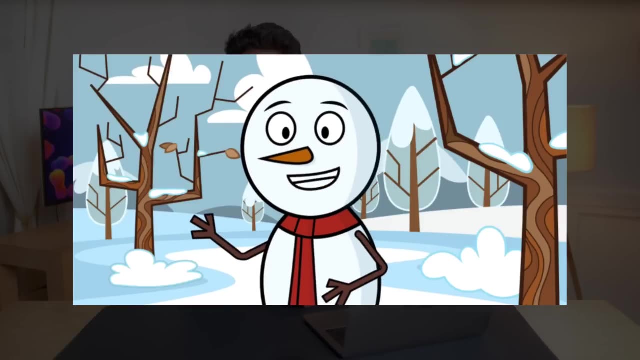 Next, let's go to the bonus part of this video, Where we'll see how you can create an animated character- that, too, with your own voice. like this: What if I told you that we can easily convert a simple sentence, or even a paragraph, into an eye-catching animation video? 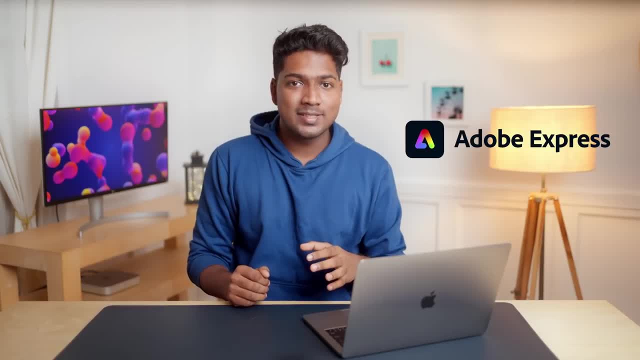 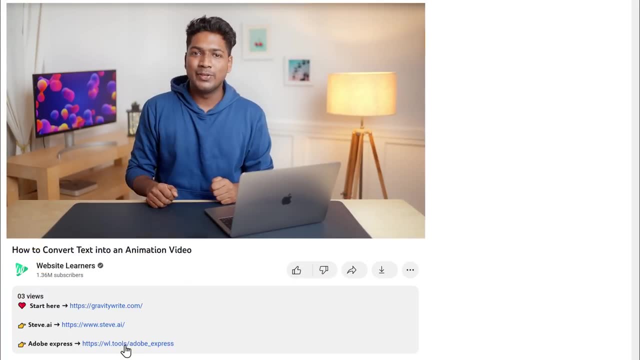 It's very simple. we're going to use a tool called Adobe Express and using this tool, let's create our very own animated character in just a matter of seconds. To do that, just click the link below this video and it'll take you to the Adobe Express website. 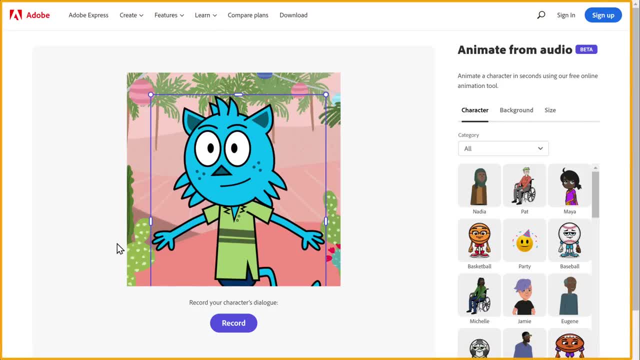 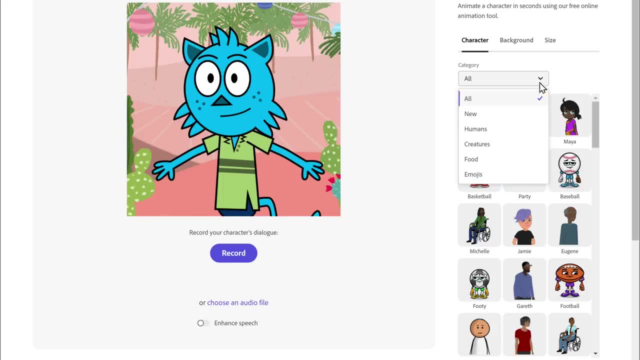 Now click on make animation and it'll take you to this page And you can choose an animated character from here. Now, if you click here, you'll find different categories to choose from. I'm going to choose creatures. You can select the one you want from all these characters. 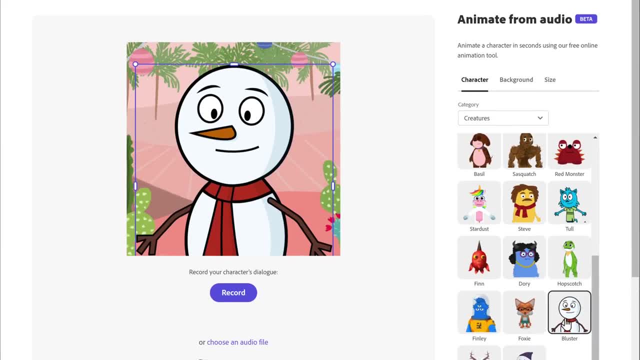 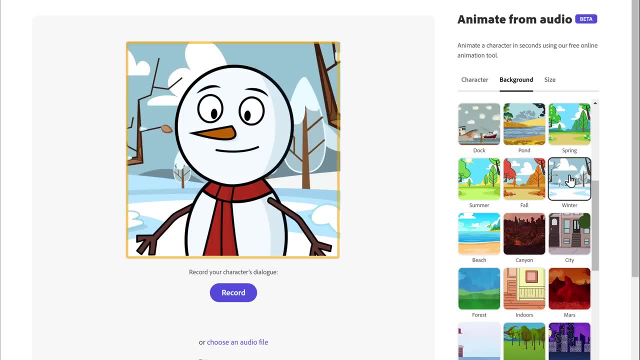 I'm going to choose this one. Once you have done that, let's add a background image for your character. So just click on background, select the one you like and it'll be applied here. Okay, next let's choose the size of our animated video. 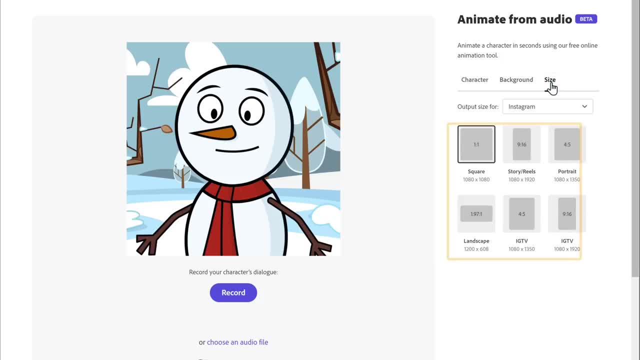 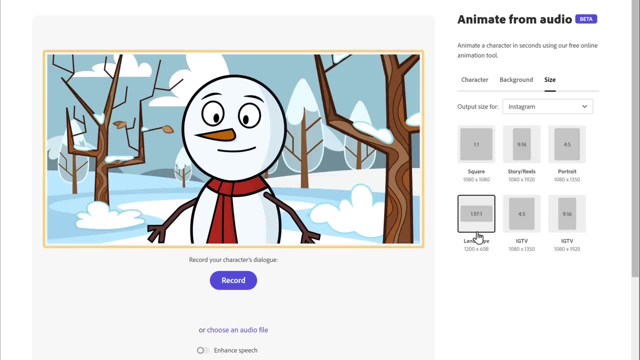 So just click on size, So select the one you want. I'm going to select this one. Okay, so now our animated character is ready. Next, let's add our voice to this animated character. Here you can see that we have two different options. 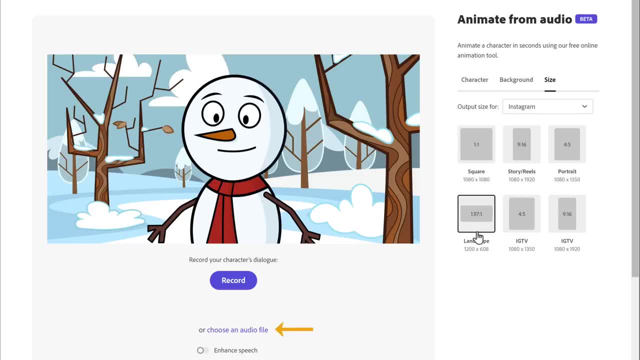 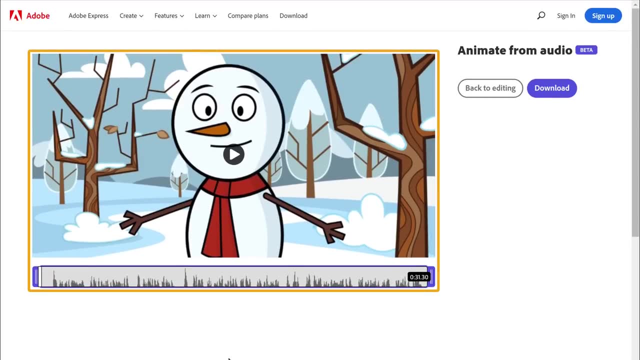 So you can either add your own voice by recording it live or by uploading an audio file. I'm going to upload an audio file. Select your audio file. We have successfully created an animated character with our own voice. Now, if you play it, you can see the preview of our video. 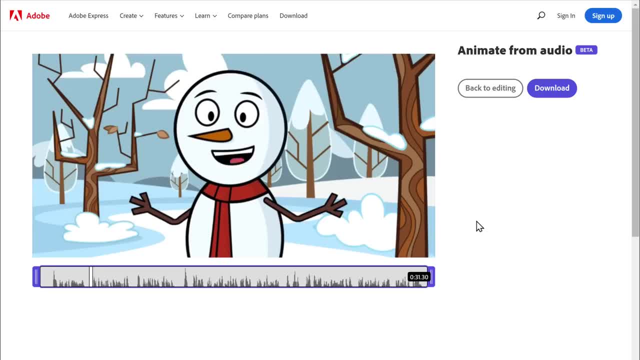 Are you curious to make your own animation videos, but you find it too complicated or time consuming to create one. Well, what if I told you that we can easily convert a simple sentence, or even a paragraph, into an eye-catching animation video. If everything looks good, you can download it by clicking here.